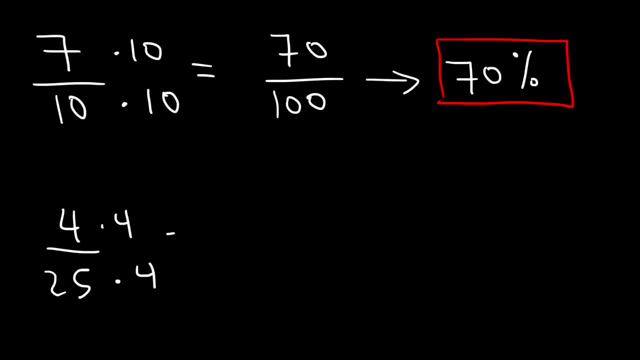 Well, 25 is 4.. So we've got to multiply the top and the bottom by 4.. So 25 times 4 is 100.. 4 times 4 is 16.. So 4 over 25 is equal to 16%. 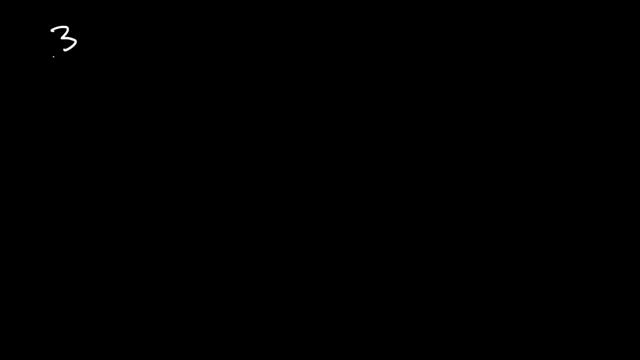 Here are some other examples. you could try 3 over 4 and 7 over 20.. Convert those into a percentage, So 3 over 4.. We know that 100 divided by 4.. We know that 100 divided by 4.. 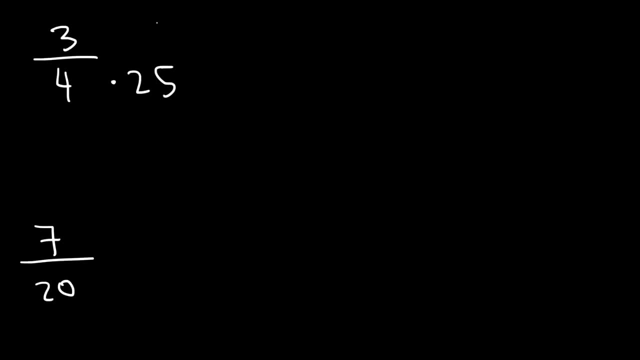 We know that 100 divided by 4 is 25.. So to get a denominator of 100, we've got to multiply the top and the bottom by 25.. 4 times 25 is 100.. 3 times 25 is 75.. 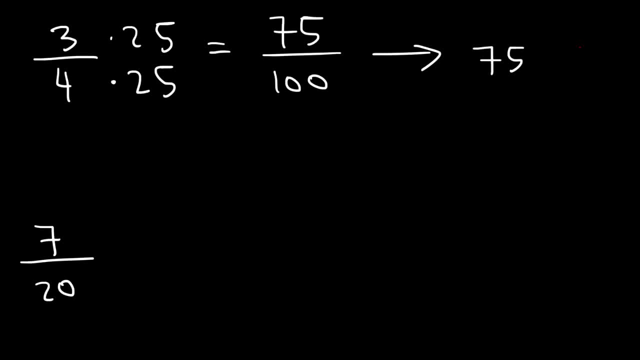 So this corresponds to 75%. Now, 100 divided by 20 is 5.. So for the second fraction, you want to multiply the top and the bottom by 5.. 20 times 5 is 100.. 7 times 5 is 35.. 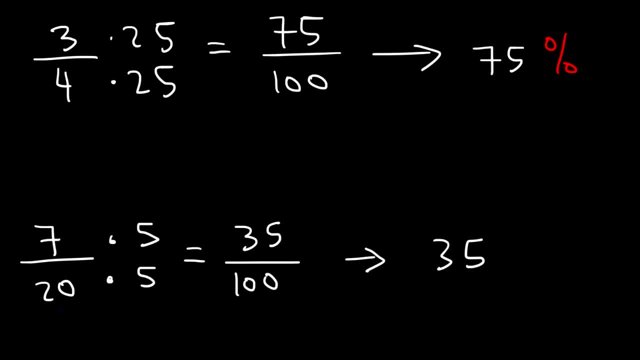 So the answer is 35%. So that's the first method in which you can convert a fraction into a percentage. But now what about something like 3 over 8? 8 doesn't go into 100 nicely, So we're going to use a different method. 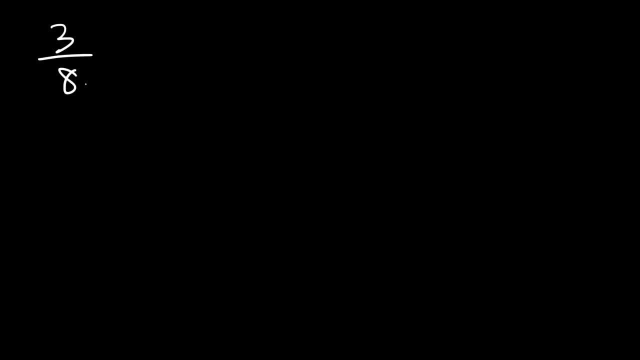 We're going to convert the fraction into a decimal and then convert the decimal into a percent. One way to convert a fraction into a decimal is to use long division. So 8 doesn't go into 3 nicely, So what we need to do is add a 0.. 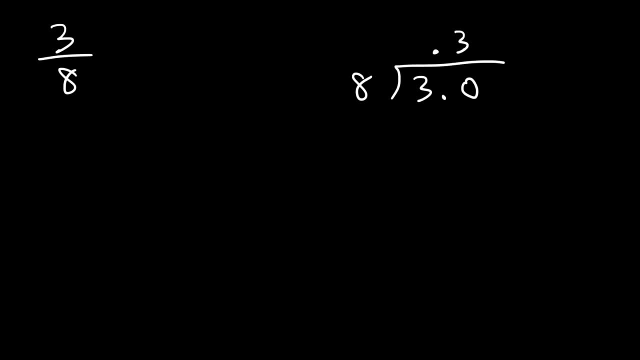 8 goes into 30. three times 8 times 3 is 24.. We're going to treat 3.0 as if it's 30. It's really supposed to be 2.4.. Now, 30 minus 24 is 6.. 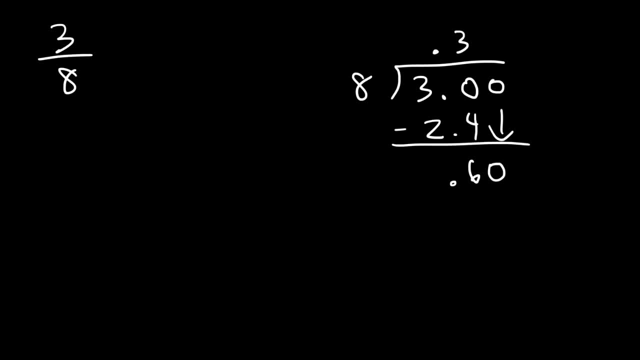 So we're going to add a 0.. Now, how many times does 8 go into 60?? 8 times 7 is 56. But 8 times 8 is 6. So 8 times 6 is 64.. 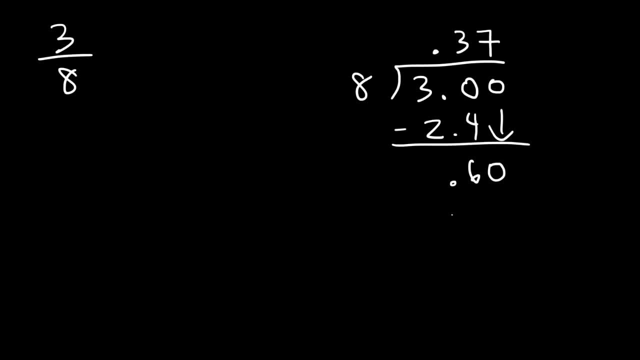 Which exceeds 60. So 8 goes into 60 seven times And it's going to be 56.. 60 minus 56 is 4.. And let's add another 0. Now 8 goes into 40. nicely, It goes into it 5 times. 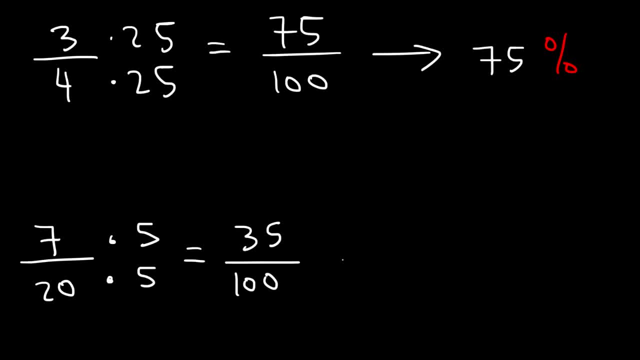 20 times 5 is 100.. 7 times 5 is 35.. So the answer is 35%. So that's the first method in which you can convert a fraction into a percentage. But now what about something like 3 over 8?? 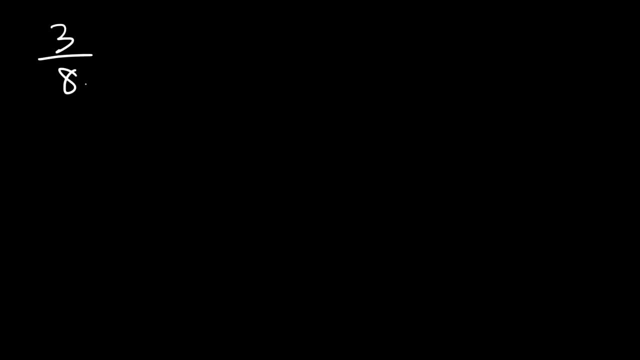 8 doesn't go into 100 nicely, So we're going to use a different method. We're going to convert the fraction into a decimal and then convert the decimal into a percent. One way to convert a fraction into a decimal is to use long division. 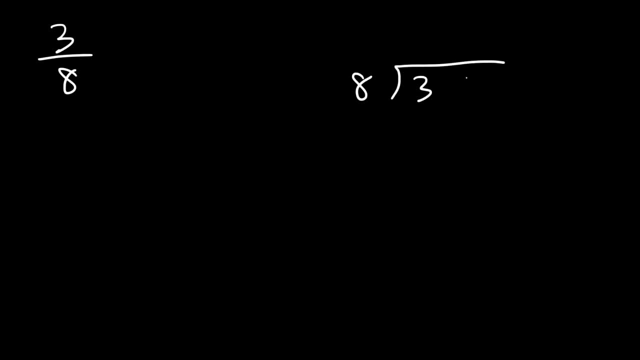 So 8 doesn't go into 3 nicely, So what we need to do is add a 0.. 8 goes into 30. three times 8 times 3 is 24.. We're going to treat 3.0 as if it's 30.. 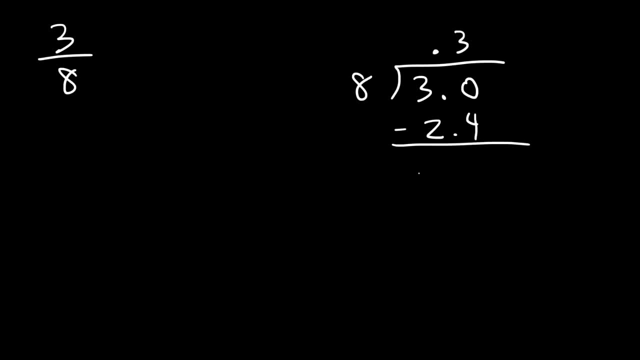 It's really supposed to be 2.4.. Now, 30 minus 24 is 6.. So we're going to add a 0.. Now, how many times does 8 go into 60?? 8 times 7 is 56.. 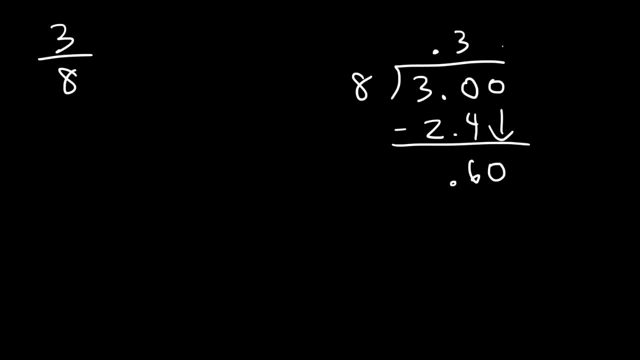 But 8 times 8 is 64, which exceeds 60. So 8 goes into 60 seven times And it's going to be 56.. 60 minus 56 is 4.. And let's add another 0.. 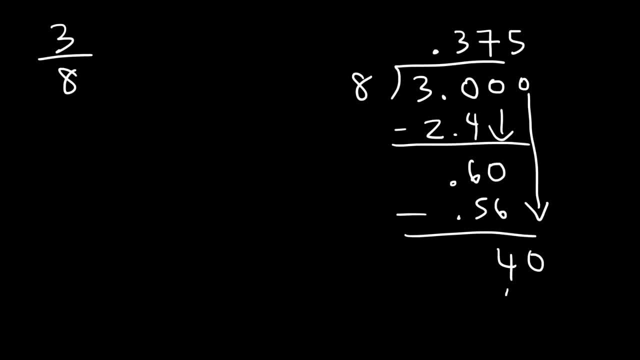 Now 8 goes into 40. nicely, It goes into it five times, So now we no longer have a remainder. So 3 over 8 is basically .375 as a decimal. Now how can we convert this decimal value to a percentage? 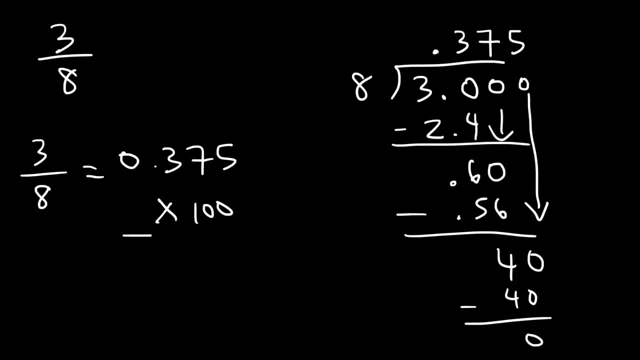 In order to do that, multiply it by 100.. .375 times 100,: all you've got to do is move the decimal 0.2 units to the right. That's 37.5%. So that's the second way in which you can convert a fraction into a percentage. 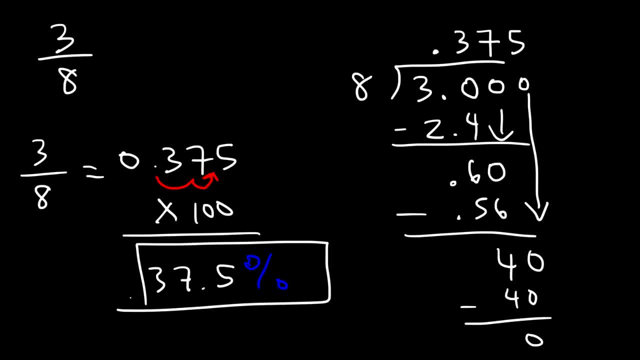 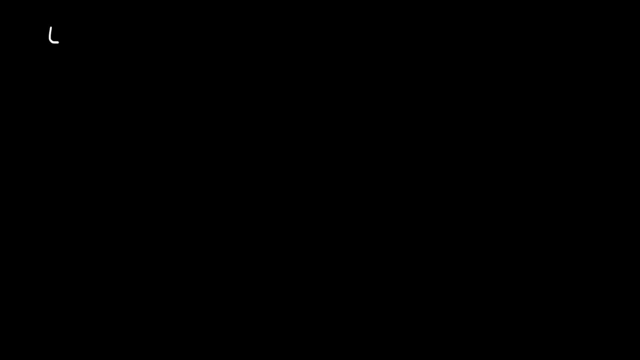 Use long division to convert it to a decimal, and then multiply the decimal by 100, and then you'll have the percentage. Now let's try another example. Let's convert 4 over 7 into a percentage, But we need to convert it to a decimal first. 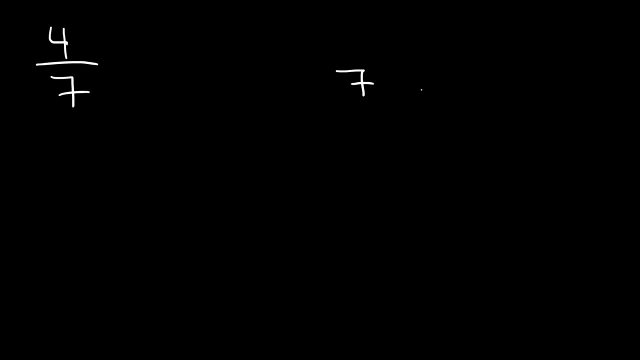 So let's use long division. We're going to put the 7 on the outside and the 4 on the inside. Now 7 doesn't go into 4.. So we need to add a 0.. Now how many times does 7 go into 40?? 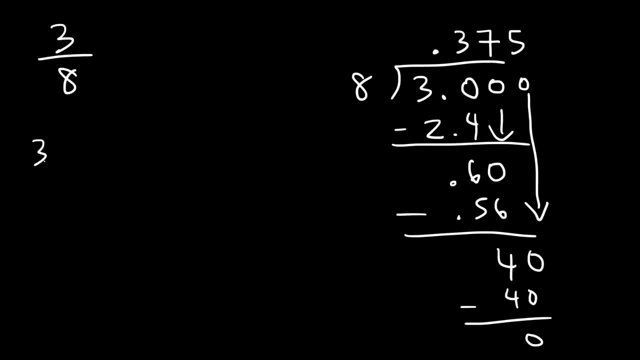 So now we no longer have a remainder. So 3 over 8 is basically .375 as a decimal. Now how can we convert this decimal value to a percentage? In order to do that, we're going to multiply by 100.. .375 times 100.. 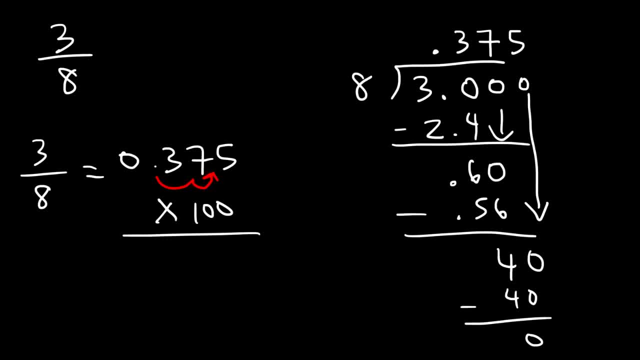 All you got to do is move the decimal .2 units to the right. That's 37.5%. So that's the second way in which you can convert a fraction into a percentage Use long division to convert it to a decimal And then multiply the decimal by 100.. 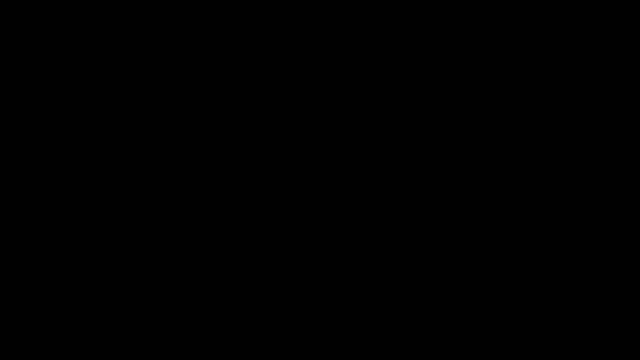 And then you'll have the percentage. Now let's try another example. Let's convert 4 over 70.. 4 over 7 into a percentage, But we need to convert it to a decimal first, So let's use long division. 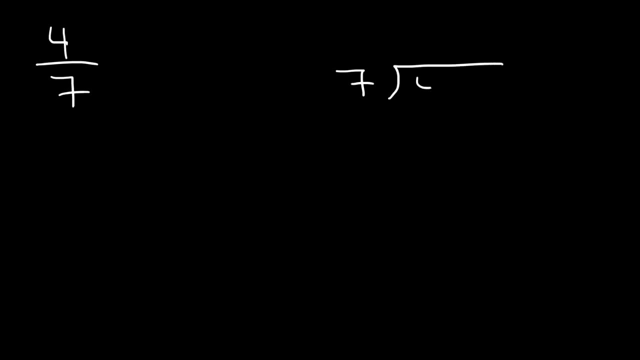 We're going to put the 7 on the outside And the 4 on the inside. Now, 7 doesn't go into 4.. So we need to add a 0.. Now how many times does 7 go into 40?? 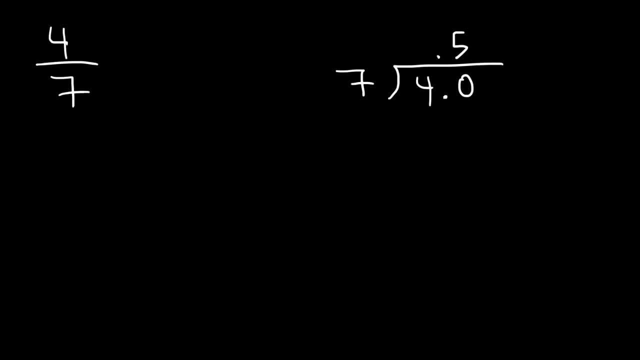 7 goes into 40 5 times. 7 times 5 is 35. And 40 minus 35 is 5.. Now we need to add another 0.. How many times does 7 go into 50?? 7 goes into 50 7 times. 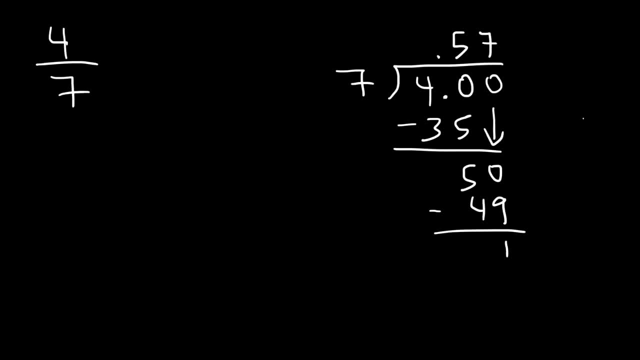 7 times 7 is 49. With a difference of 1.. And then we can add another 0.. 7 goes into 10 one time. 7 times 1 is 7.. 10 minus 7 is 3.. 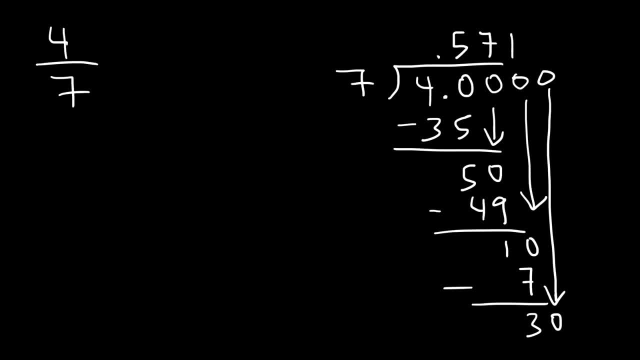 And then if we add another 0, that's 30.. 7 goes into 30 4 times, With a remainder of 2.. But that's enough. We can round it to the nearest thousandth place. So 4 over 7 is about 0.571.. 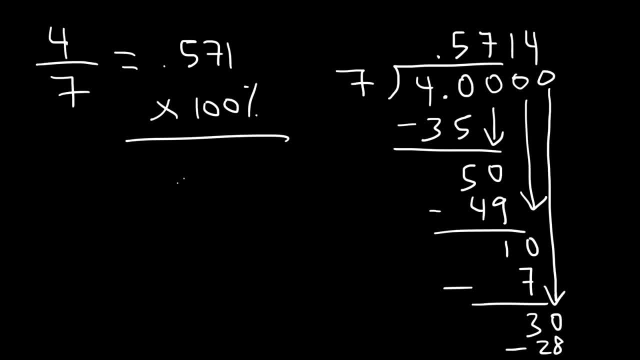 Now, if we multiply that by 100. This will give us about 57.1% As a rounded answer Which we can work with. So that's how you can convert the fraction 4 over 7 into a percentage. Now what about converting a mixed fraction into a percentage? 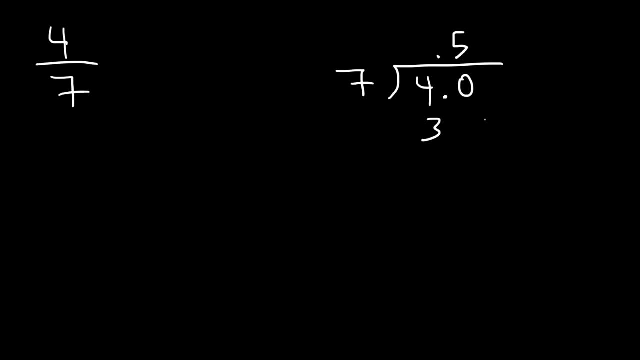 7 goes into 40. five times 7 times 5 is 35. And 4.. 40 minus 35 is 5.. Now we need to add another 0.. How many times does 7 go into 50?? 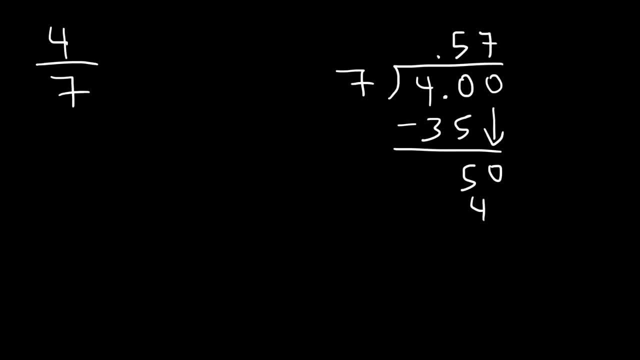 7 goes into 50. seven times 7 times 7 is 49.. With a difference: of 1.. And then we can add another 0.. 7 goes into 10. one time. 7 times 1 is 7.. 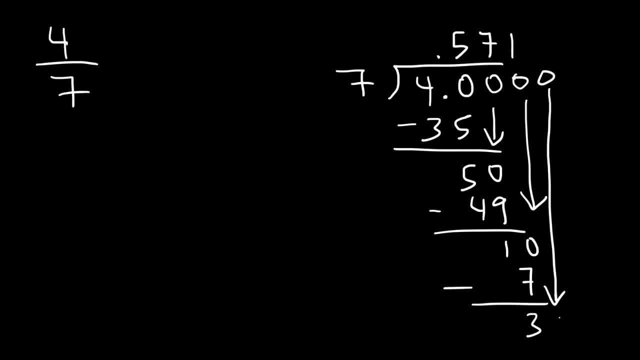 10 minus 7 is 3.. And then, if we add another 0, that's 30.. 7 goes into 30 four times, With a remainder of 2.. But that's enough. We can round it to the nearest thousandth place. 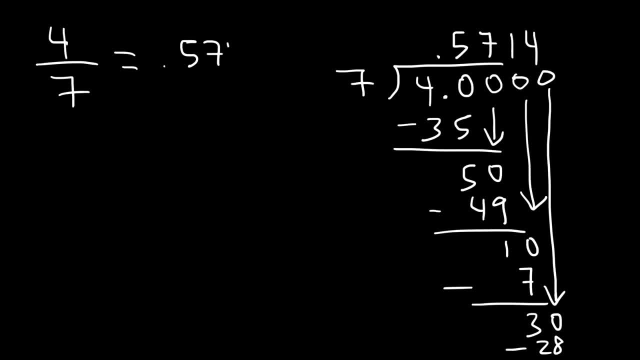 So 4 over 7 is about 0.571.. Now, if we multiply that by 100, this will give us about 57.1% as a rounded answer Which we can work with. So that's how you can convert the fraction 4 over 7 into a percentage. 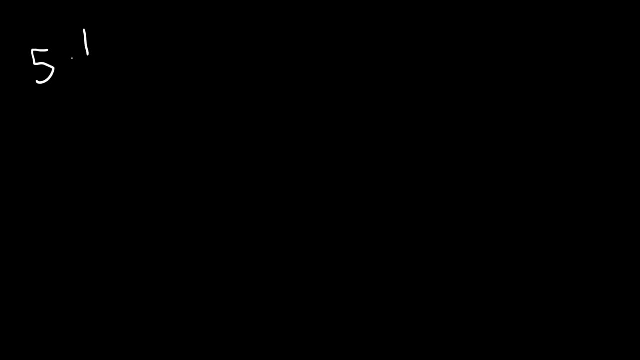 Now, what about converting a mixed fraction into a percentage? What's 5 and 1 set? What's 6 as a percentage? Well, first let's focus on the number 1 over 6.. Let's convert that into a percentage. 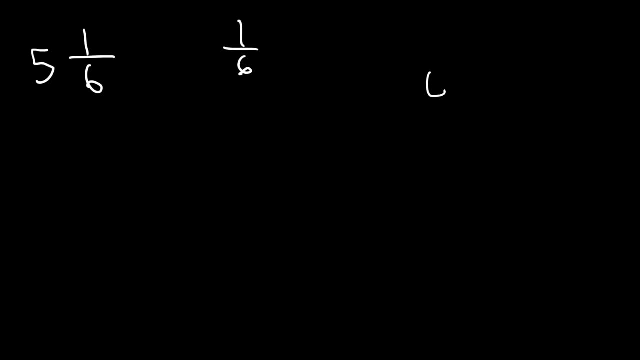 So let's use long division. 6 doesn't go into a 1, so let's add a 0.. Now 6 goes into 10 one time. 10 minus 6 is 4.. And if we add a 0,. 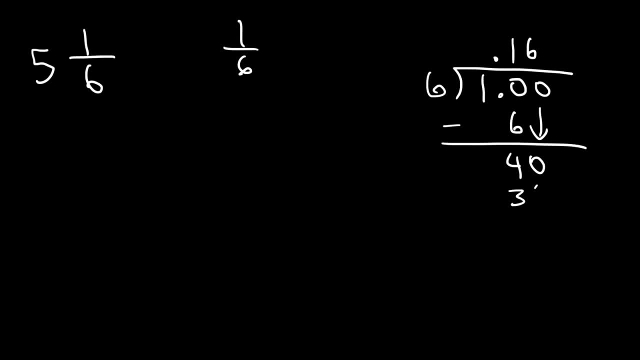 6 goes into 40 six times. 6 times 6 is 36.. And 40 minus 36 is 4.. Now let's add another 0.. 6 goes into 40 six times And notice that this process will keep repeating. 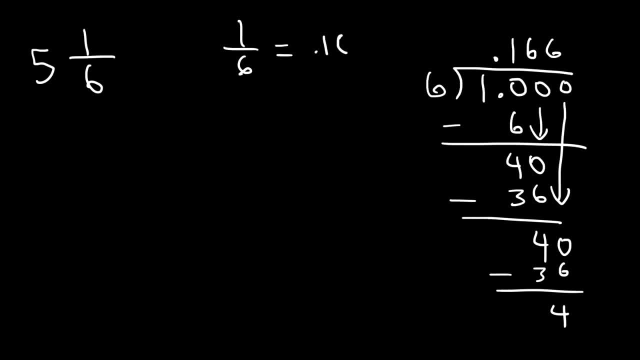 So therefore, 1 over 6 is 0.16, with the 6 repeating. So if you want to round it, you can say it's about 0.167.. Now we need to convert 0.167 into. well, actually we're not going to convert it into a percentage yet. 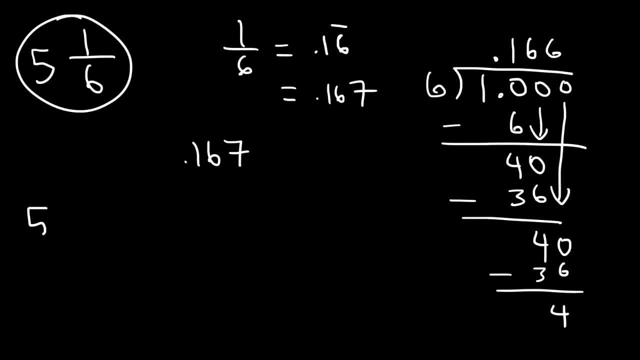 Now the number 5 and 1 six. that's basically 5 plus 1 over 6.. And 1 over 6 is about 0.167.. So the mixed fraction 5 and 1 six is 5.167.. 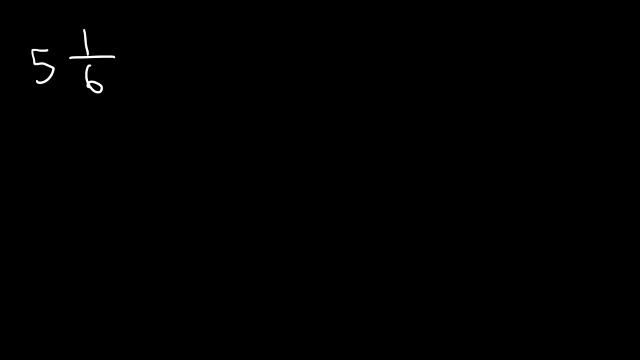 What's 5 and 1, 6 as a percentage? Well, first let's focus on the number 1 over 6.. Let's convert that into a percentage, So let's use long division. 6 doesn't go into a 1, so let's add a 0.. 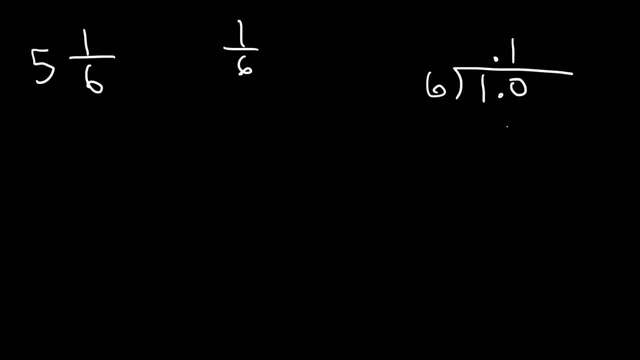 Now 6 goes into 10. one time 10 minus 6 is 4.. And if we add a 0. 6 goes into 40, 6 times 6 times 6 is 36.. And 40 minus 36 is 4.. 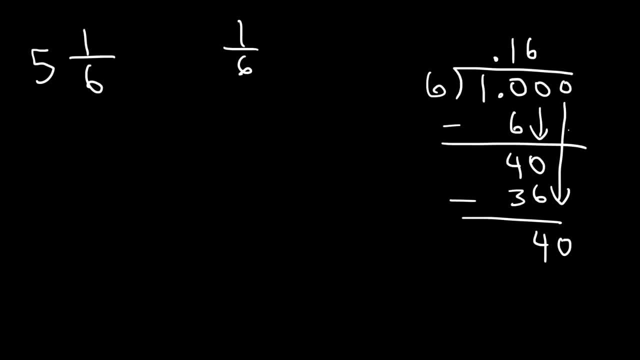 Now let's add another 0.. 6 goes into 40, 6 times And notice that this process will keep repeating. So therefore, 1 over 6 is 0.16, with the 6 repeating. So if you want to round it you can say it's about 0.167.. 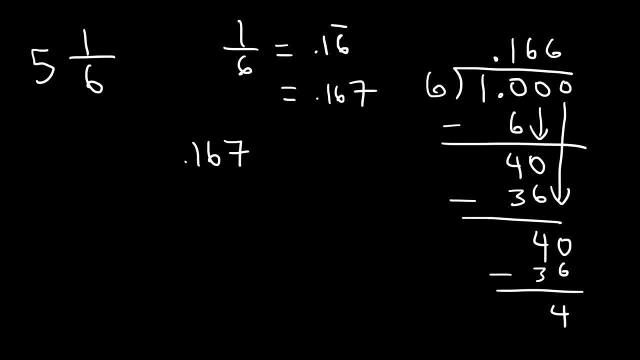 Now we need to convert 0.167.. Well, actually we're not going to convert it into a percentage yet. Now the number 5 and 1, 6.. That's basically 5 plus 1 over 6.. And 1 over 6 is about 0.167.. 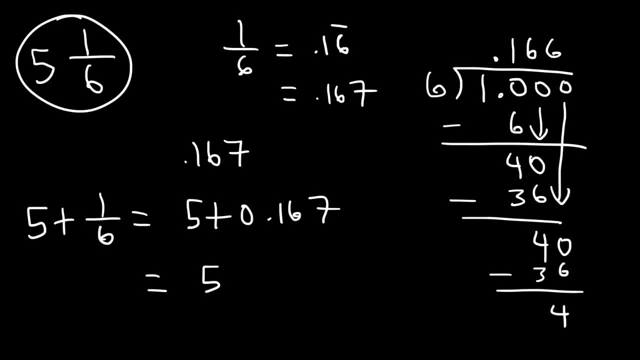 So the mixed fraction 5 and 1- 6 is 5.167.. And it is this value that we want to convert into a percentage, So we're going to multiply it by 100.. So, therefore, this fraction is equal to 516.7%. 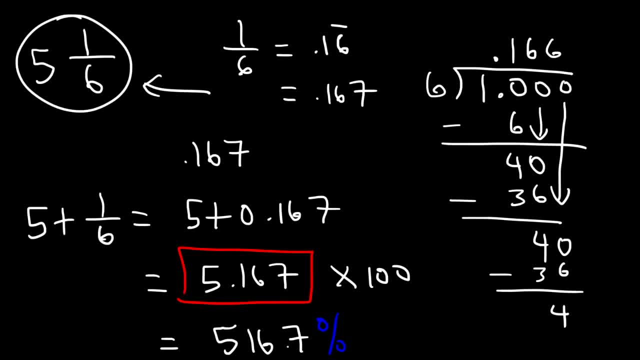 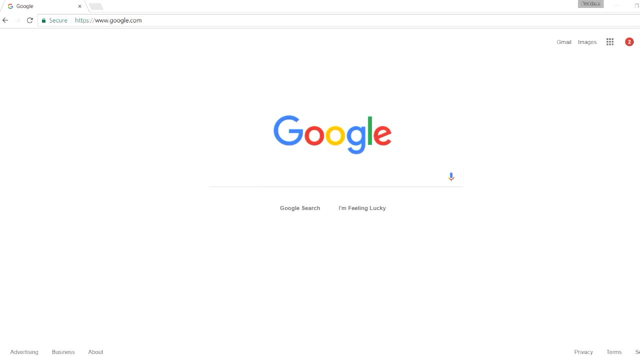 Or, if you want the exact answer, it's 516.666 repeated. Or you could just round it like this. So that's how you can convert a mixed fraction into a percentage. Now I want to show you one of my algebra courses that might be useful to you if you ever need it. 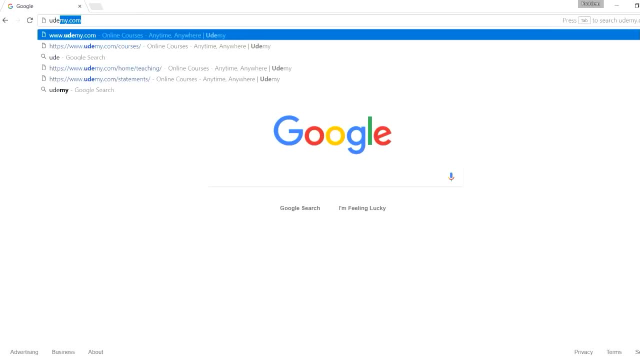 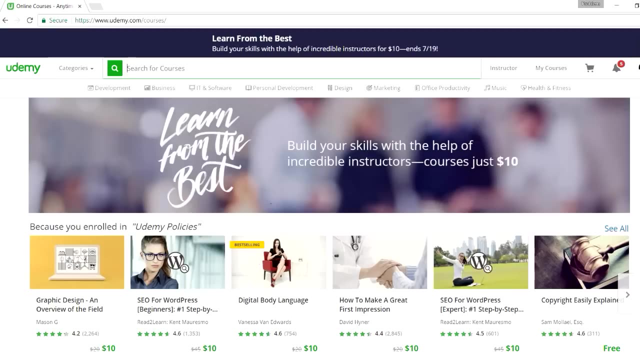 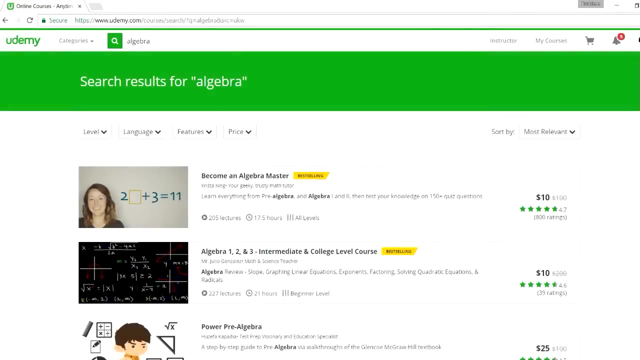 So if you want to convert a mixed fraction into a percentage, So go to udemycom Now in the search box just type in algebra And it should come up. So it's the one with the image with the black background. So if you select that option, 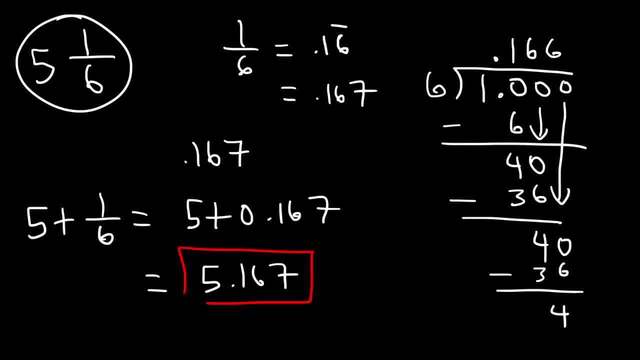 And it is this value that we want to convert into a percentage, So we're going to multiply it by 100.. So, therefore, this fraction is equal to 516.7%, Or, if you want the exact answer, it's 516.666 repeated. 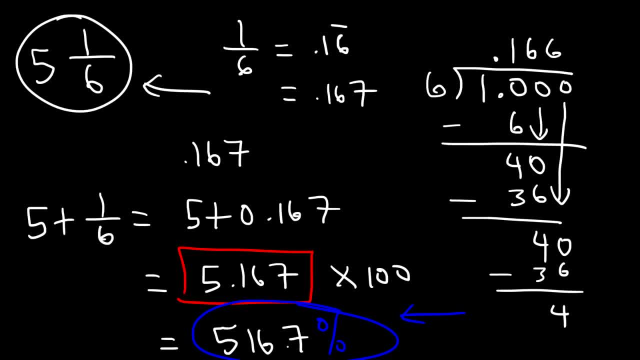 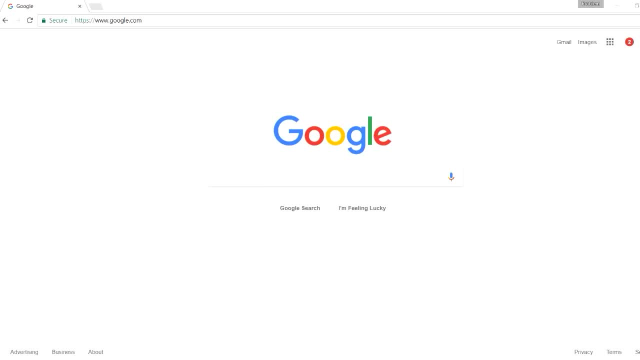 Or you could just round it like this. So that's how you can convert a mixed fraction into a percentage. Now I want to show you one of my algebra courses that might be useful to you if you ever need it. So go to udemycom. 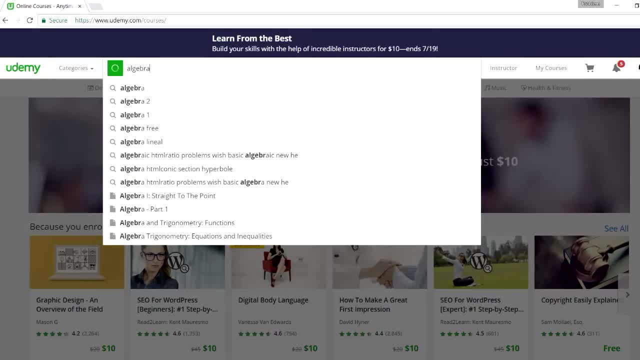 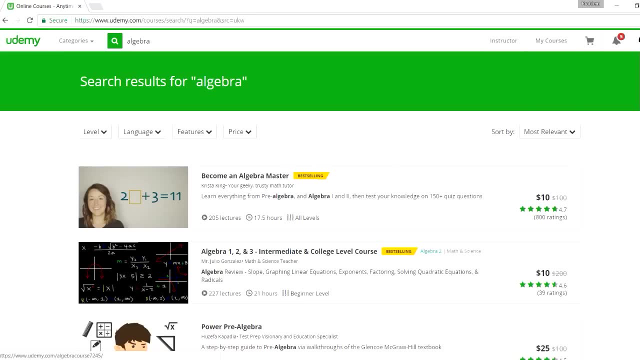 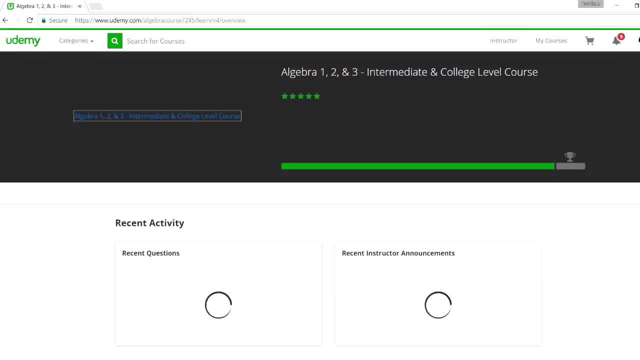 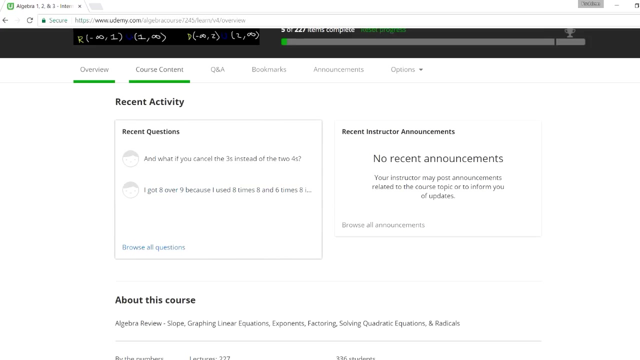 Now in the search box just type in algebra And it should come up. So it's the one with the image with the black background. So if you select that option and if you decide to go to course content, you can see what's in this particular course. 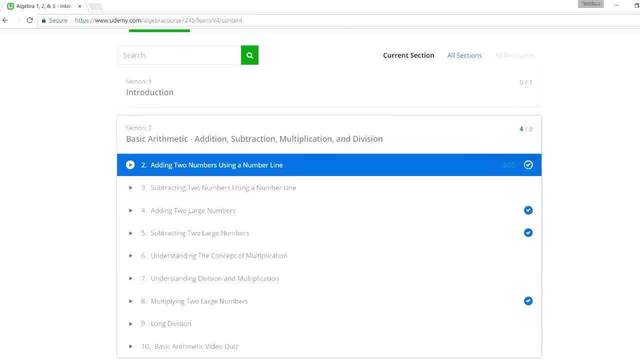 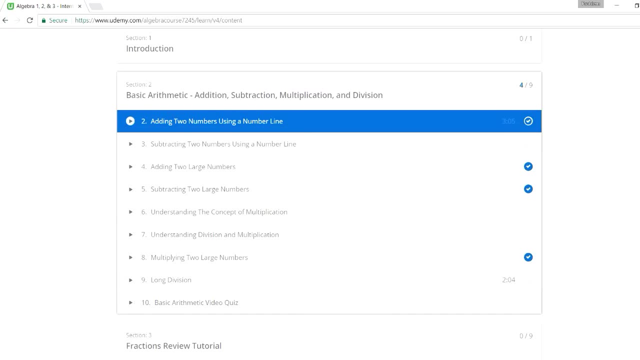 So the first section, basic arithmetic- for those of you who want to focus on addition, subtraction, multiplication and division, And it has a video quiz at the end. It's a multiple choice video quiz. You can pause it. work on the problems. 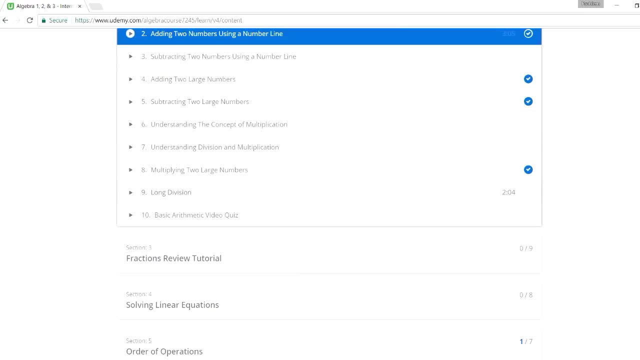 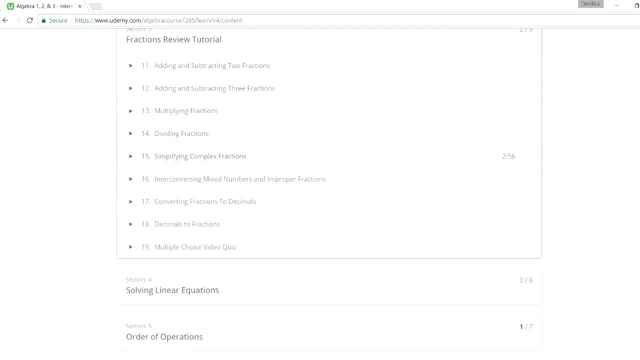 and see the solutions. It covers long division, multiplying two large numbers and things like that. The next tutorial is on fractions- Add-in subtracting fractions, multiplying and dividing fractions, converting fractions into decimals and so forth, So you can also take a look at that. 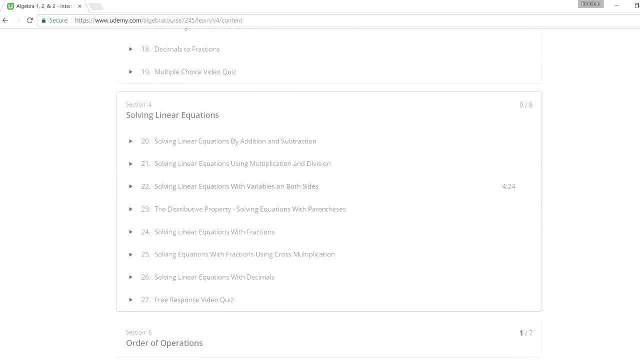 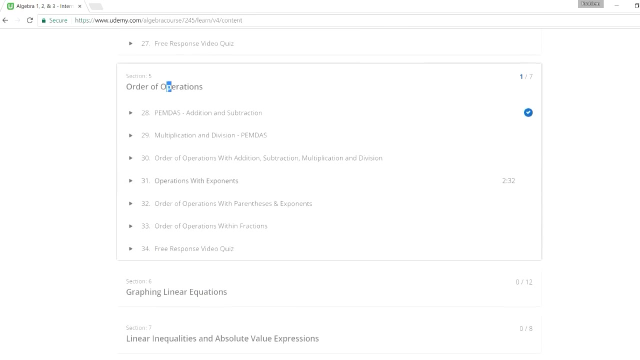 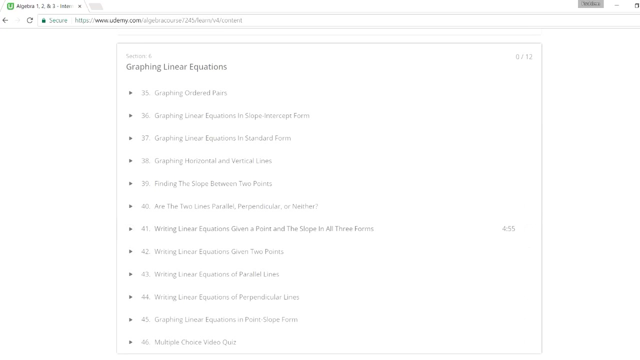 Next, solving linear equations, which we covered, And just more examples if you need more help with that. The next topic, order of operations, which is also useful, Graphing linear equations. You need to know how to calculate the slope. You need to be familiar with. 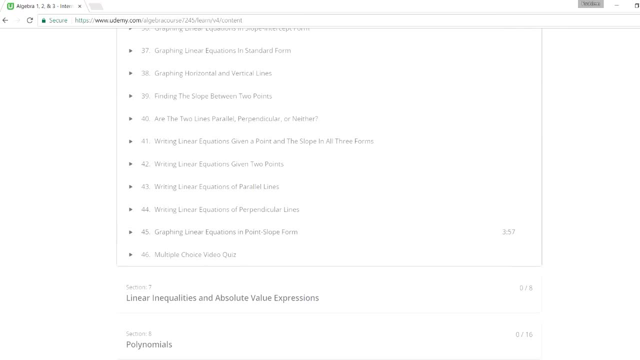 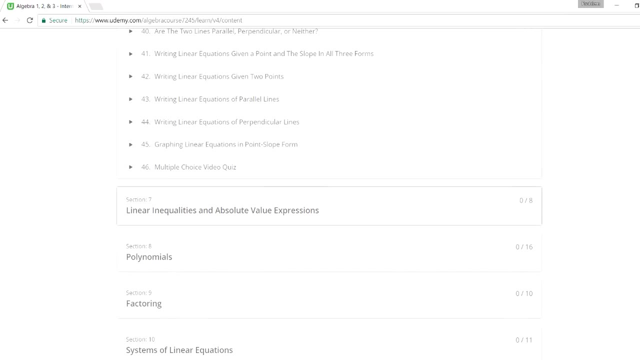 the slope, intercept form, standard form and just how to tell if lines are parallel, perpendicular and so forth, And there's a quiz that goes with that as well. The next topic is on inequalities and absolute value expressions, which are also seen. 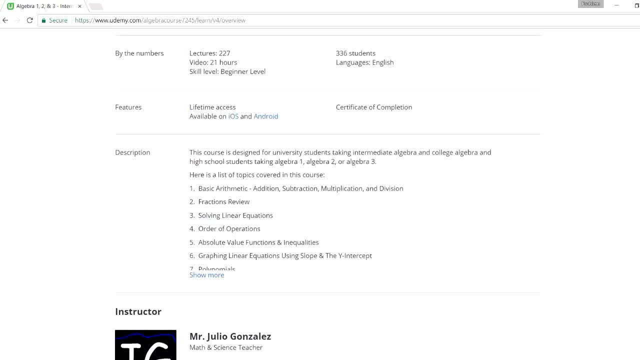 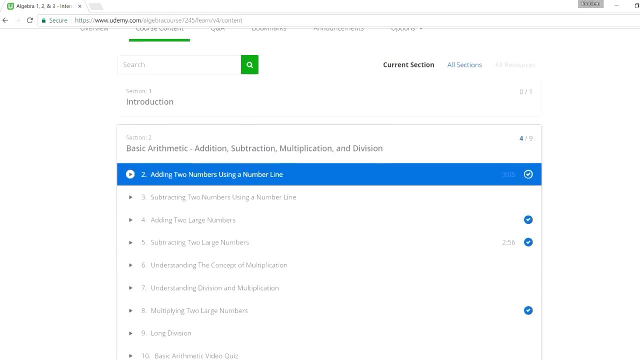 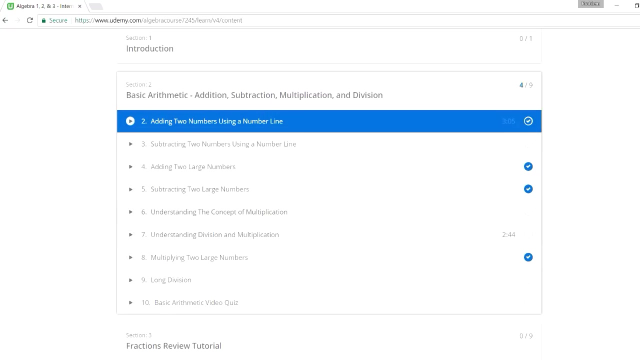 And if you decide to go to course content, You can see what's in this particular course. So the first section, basic arithmetic- For those of you who want to focus on addition, subtraction, multiplication and division, And it has a video quiz at the end. 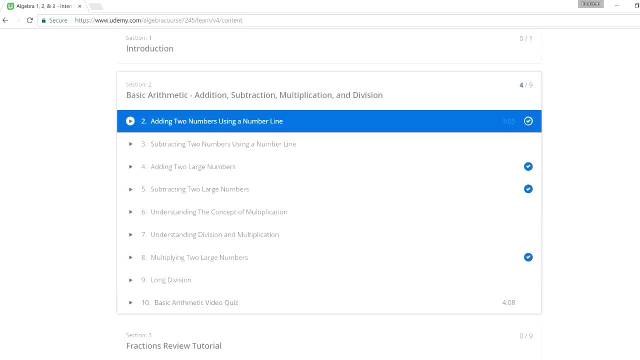 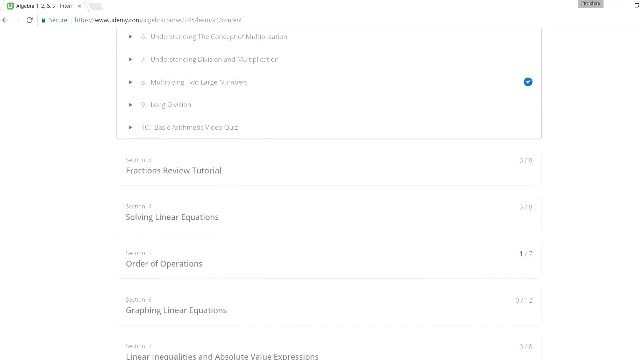 It's a multiple choice video quiz. You can pause it, work on the problems and see the solutions. It covers long division, multiplying two large numbers and things like that. The next tutorial is on fractions, Adding, subtracting fractions, multiplying and dividing fractions. 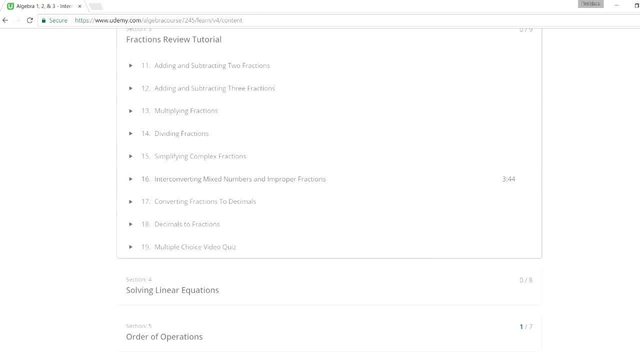 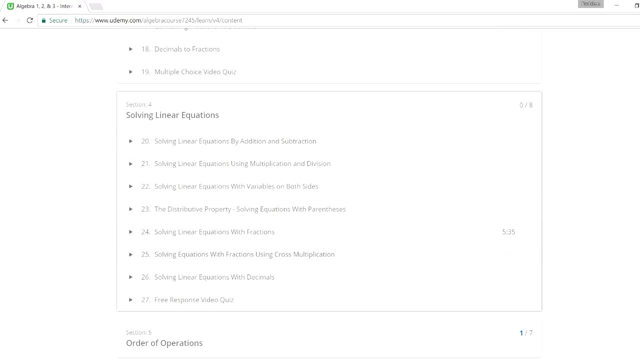 Converting fractions into decimals And so forth. So you can also take a look at that. Next, solving linear equations, which we covered, And just more examples if you need more help with that. The next topic, order of operations, Which is also useful. 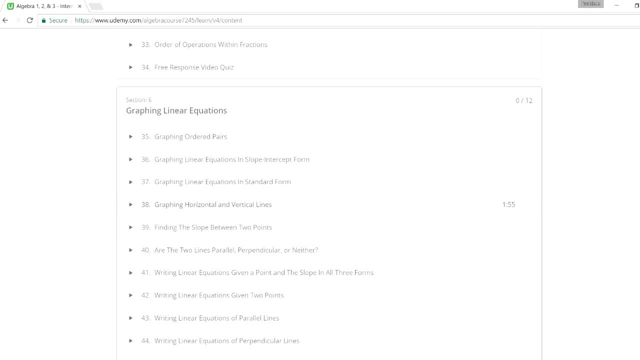 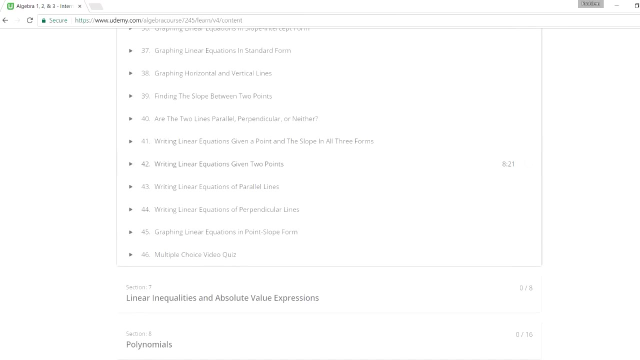 Graphing linear equations. You need to know how to calculate the slope. You need to be familiar with The slope intercept form, standard form And just how to tell if lines are parallel, perpendicular and so forth. And there's a quiz that goes with that as well. 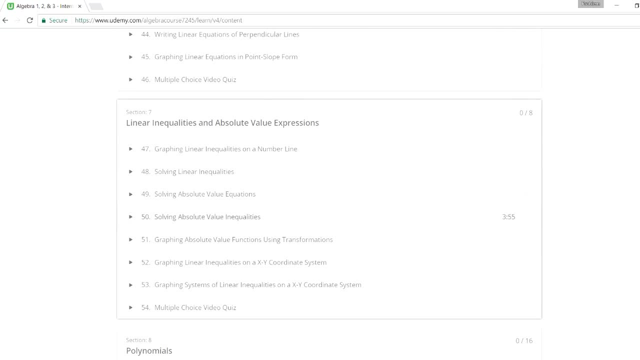 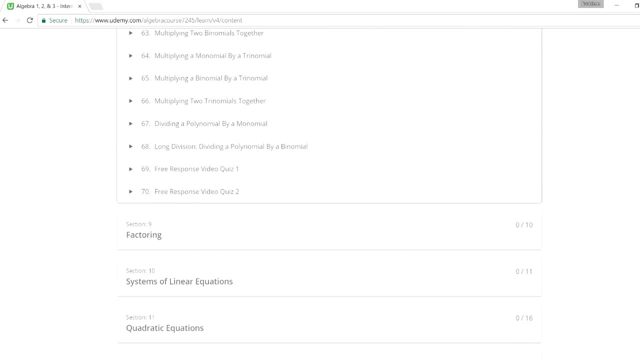 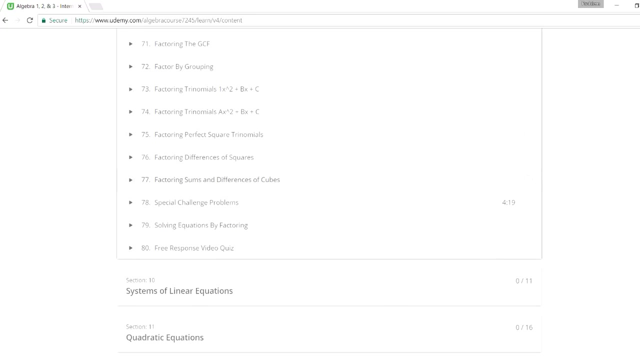 The next topic is on inequalities and absolute value expressions, Which are also seen in a typical algebra course. And then we have polynomials, And that's a long section, And then factoring- That's another topic you need to master- And then system of equations. 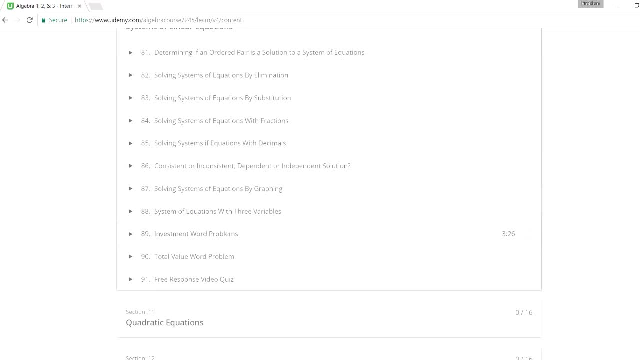 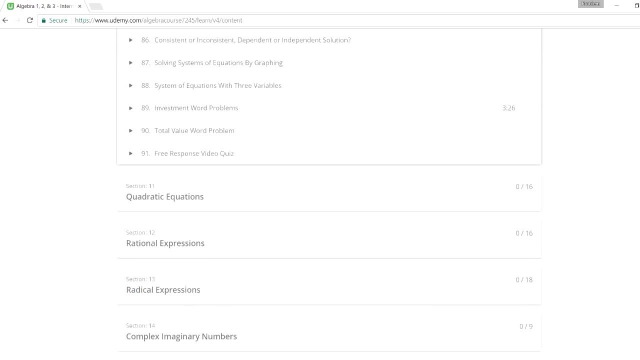 You can solve it by elimination Substitution. There's also word problems as well. Sometimes you got to solve equations with three variables- X, Y and Z. So that could be helpful. Next, quadratic equations: How to use a quadratic formula. 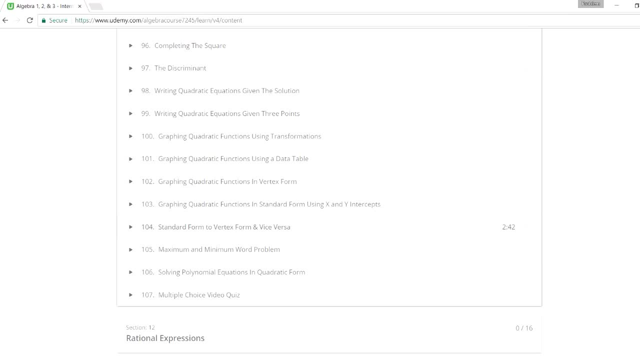 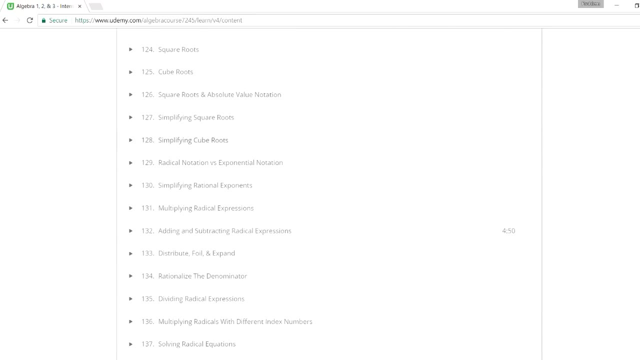 How to graph them, How to convert between standard and vertex form, And then you have rational expressions And radical expressions, Solving radical equations, Simplifying it, Things like that. And every section has a formula, And every section has a quiz. 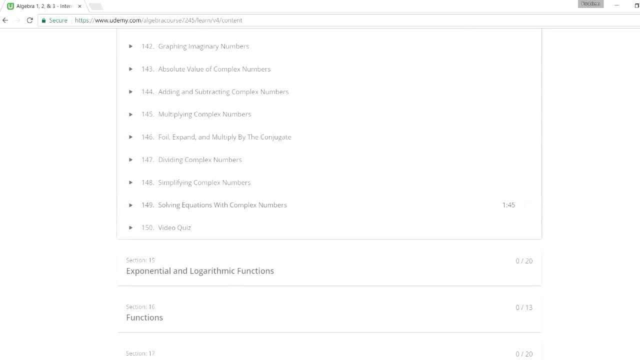 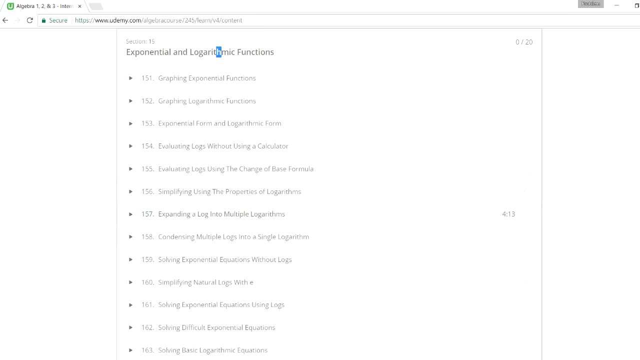 So you can always review what you've learned If you have a test the next day. So here we have complex imaginary numbers. You need to know how to simplify those Exponential Functions Logs. I have a lot of videos on logs.